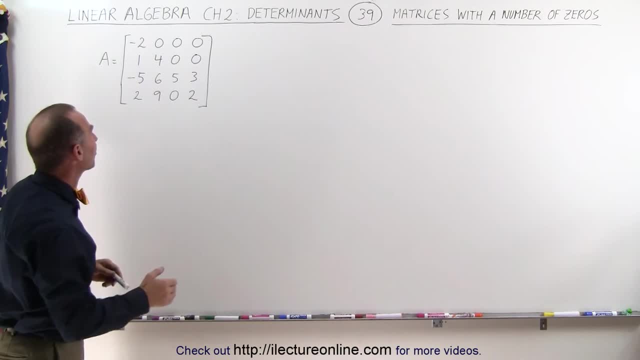 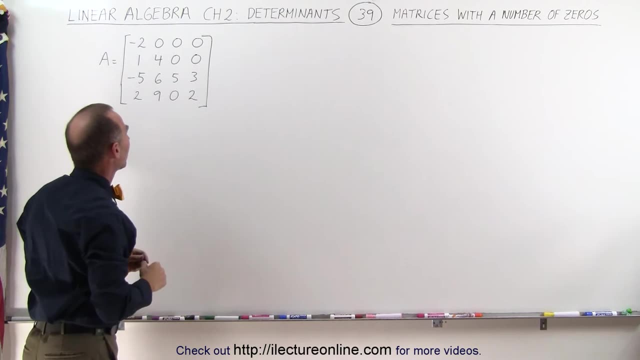 to find the determinant of this matrix. For example, if we take the top row, we have three zeros and only one of the four elements that has an actual number in it. In other words, we can ignore the other three right there. And then, if we go to the second row, also notice that we have lots. 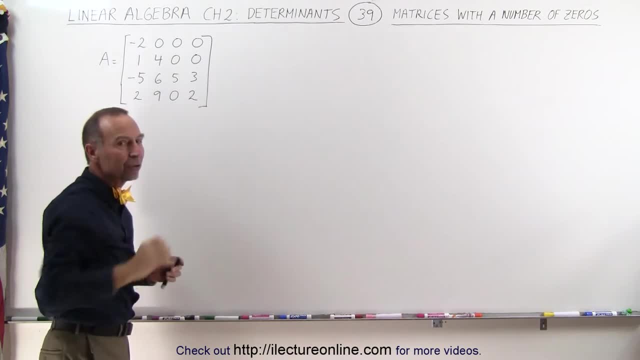 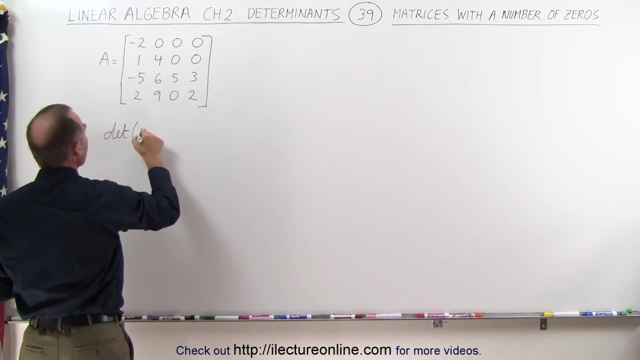 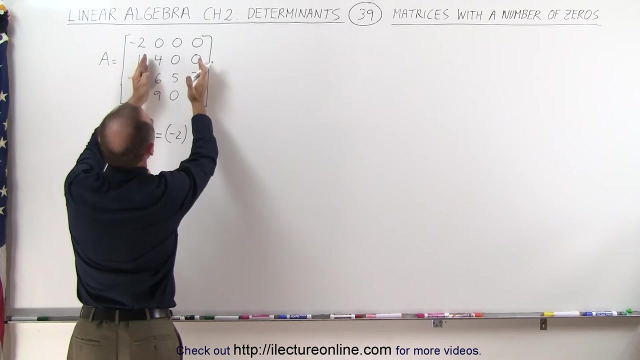 of zeros here. That means we can ignore all that and the reduction becomes fairly easy. This can then be written as follows: The determinant of A can then be written: we can take the single element right here: negative two multiply times the determinant of this matrix. 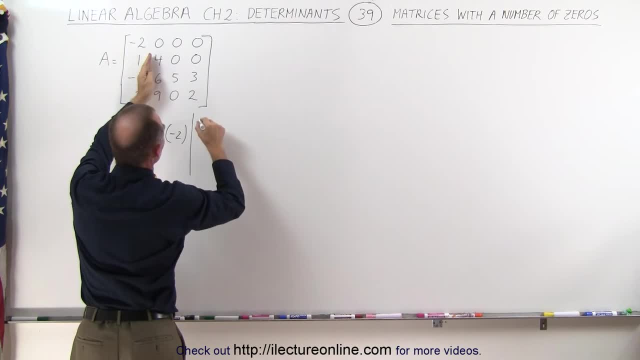 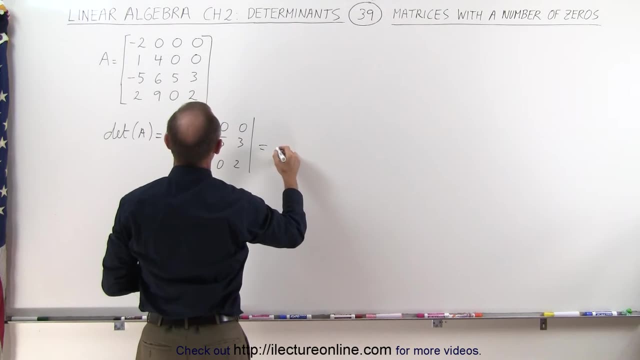 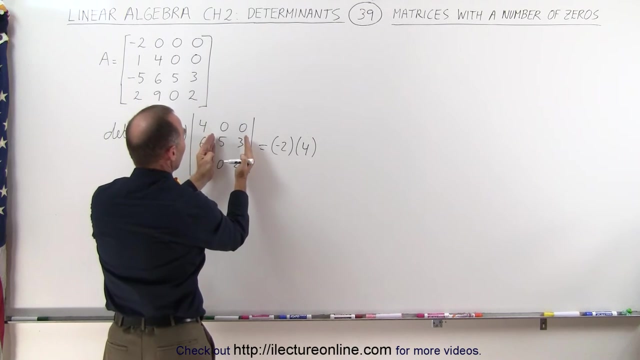 right here. right. So that's times the determinant of the matrix four, three, zero nine, zero two. But since these are zeros, that means that this can now be written to be negative two times four, and then we can cross out this row and this column and now we have this matrix, right here. 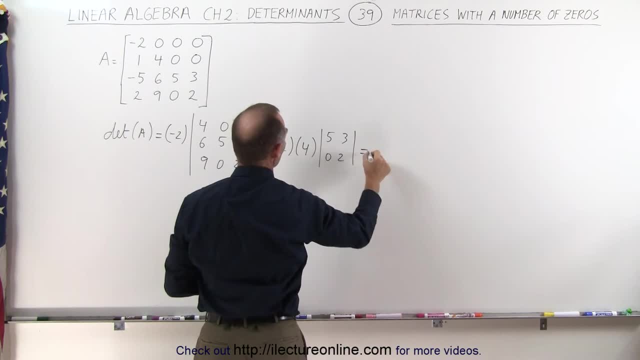 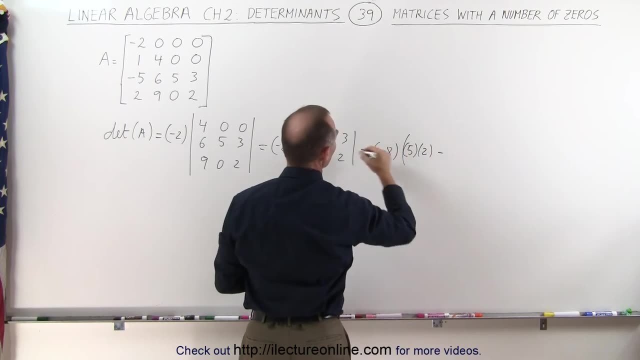 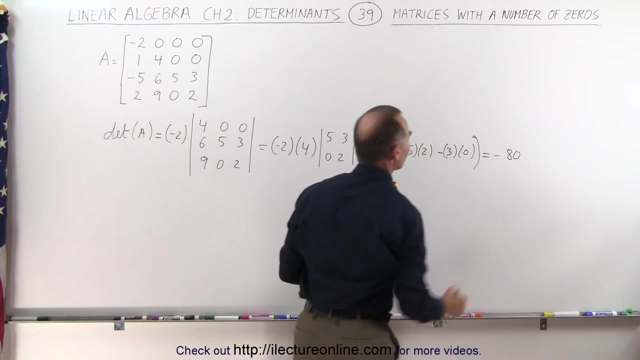 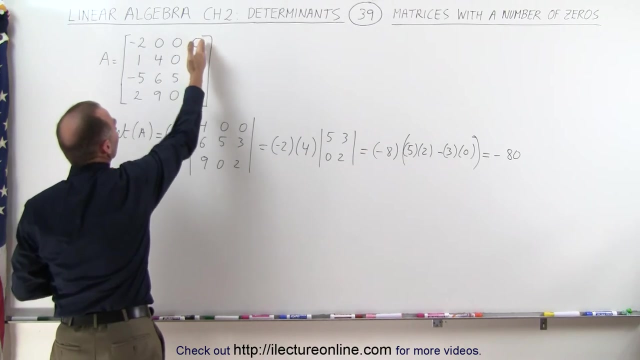 which is the matrix five, zero and two, Which essentially can be written as negative eight times five times two minus three times zero, And so we get minus eight times or minus 80, and that would be the determinant of that matrix. now we're going to do this again, but now we're going to take this column right here. 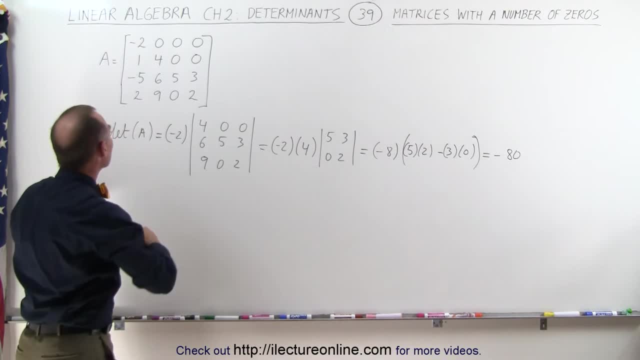 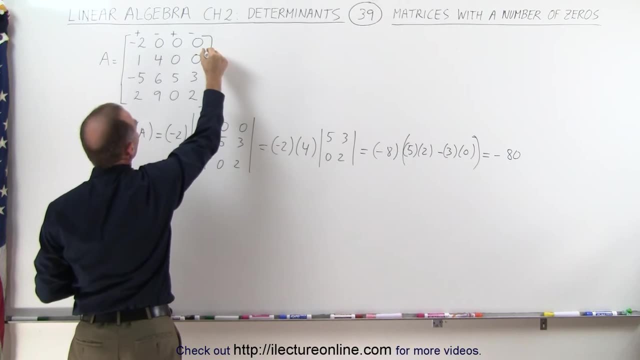 with a 4 by 4. we have to be careful about the signs. notice that the upper left corner is a plus and it alternates signs. this is a minus, a plus, a minus. we go around the corner. this is the plus, a minus and a plus. so when we then take 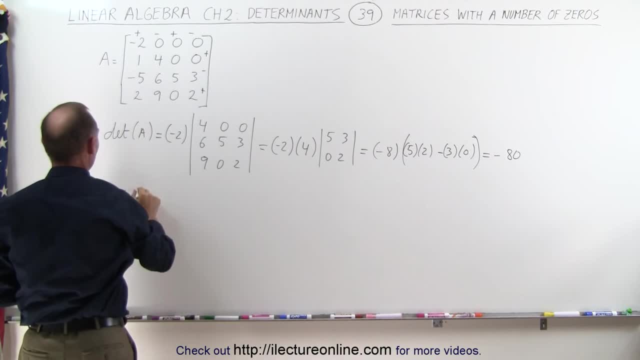 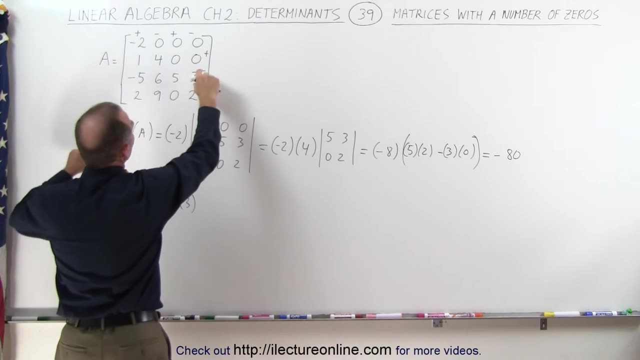 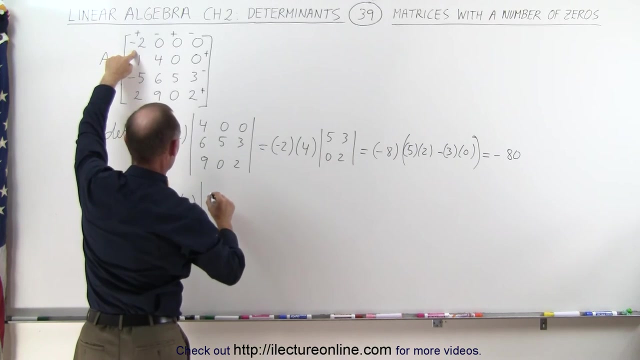 this element. right here, we can say that the determinant of the matrix a is equal to negative times 3, and now, when we take that, we have this, these nine elements remaining to give us a 3 by 3 matrix. so we have a minus 2, 0, 0, 0, 1 and we have 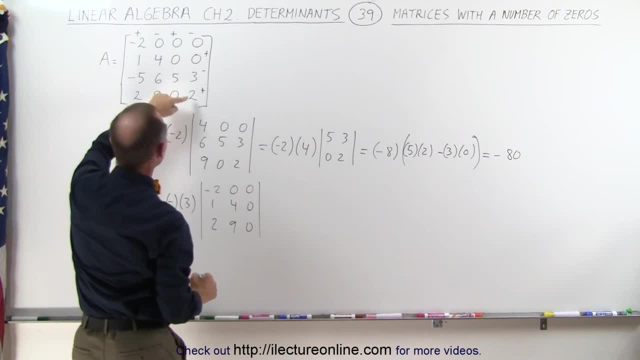 the 2, 1, 9 and 0, and then we take this one right here, so it would be plus 2 times the matrix if we cross out this 1 and we take this one right here, so it would be plus 2 times the matrix if we.